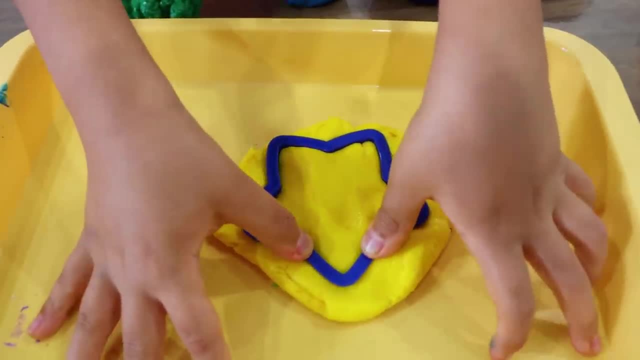 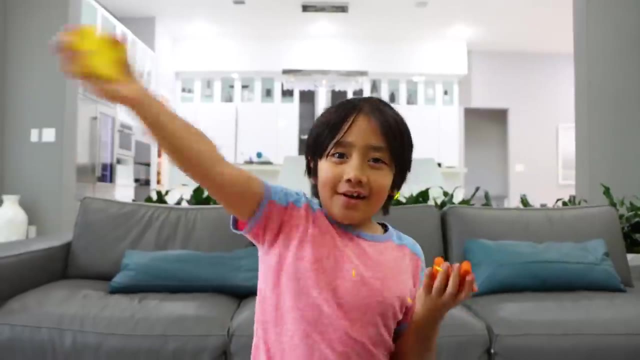 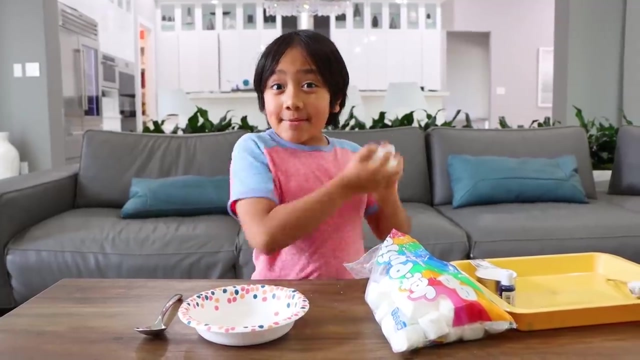 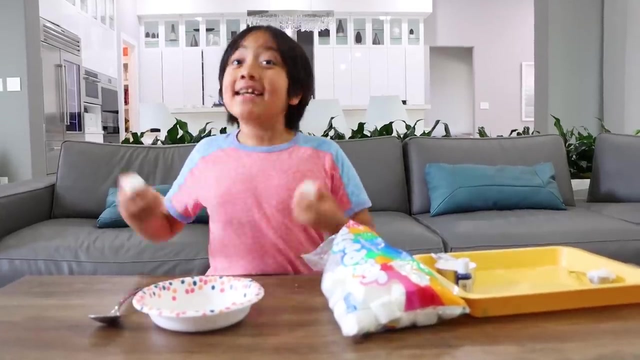 Okay, push it in Nice. What do you guys wish for? Shooting star. Welcome to Ryan's World. Hey guys, today I'm going to make a homemade plano with marshmallows. First thing you're going to need is marshmallows. Here I'm going to use 10 marshmallows. 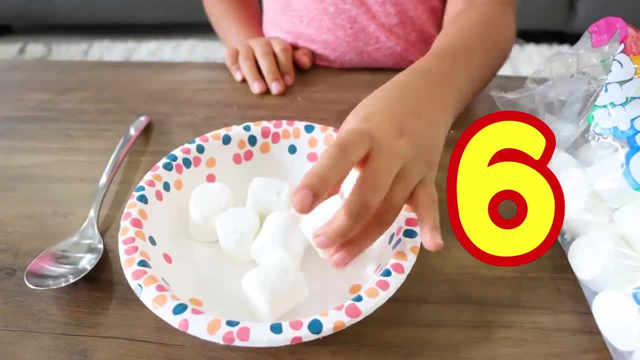 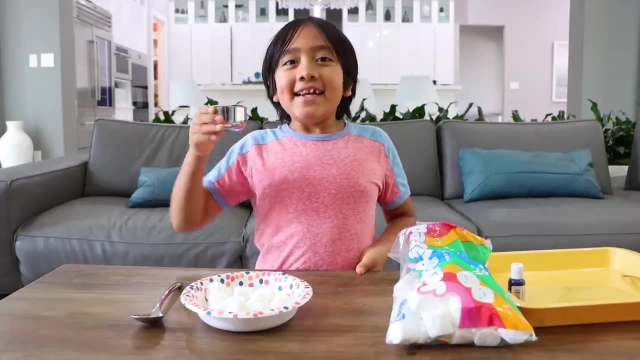 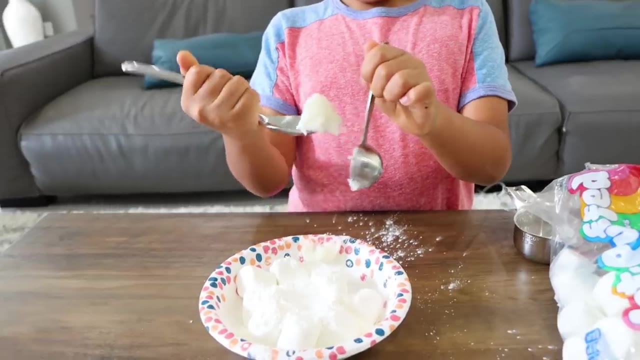 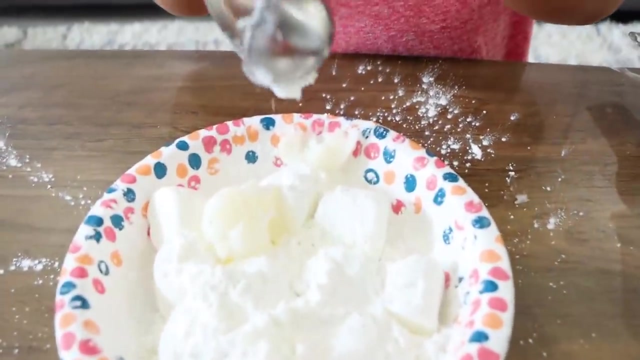 Five already, Six, seven, eight, nine and ten. Next thing you need is half a cup of cornstarch. Next is one tablespoon of coconut oil And there, Next thing, ask your grown-up to microwave this for 30 seconds. 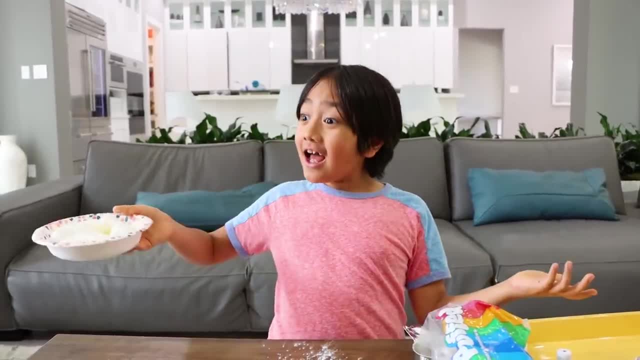 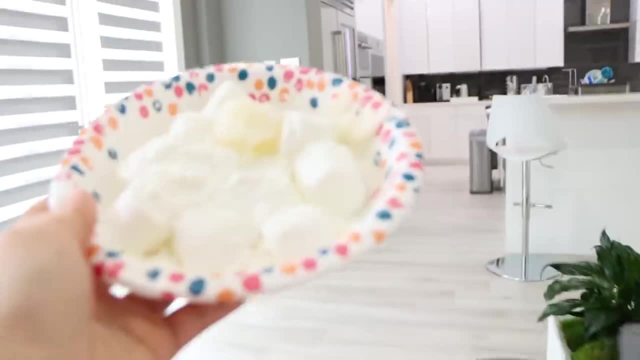 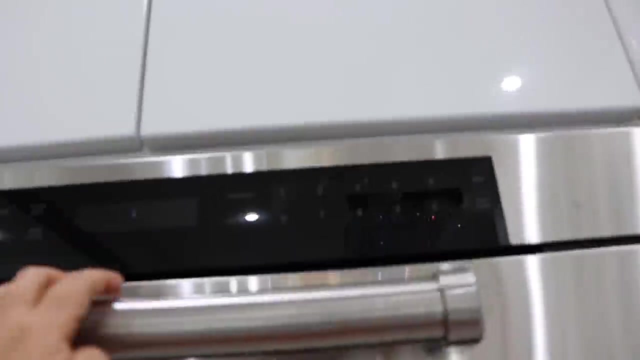 Can you microwave this for 30 seconds? Of course, Ryan, I'm right here. Thank you, Be right back. Okay, taking this to the microwave: Opened Microwave- 30 seconds, Okay. and if you look here, 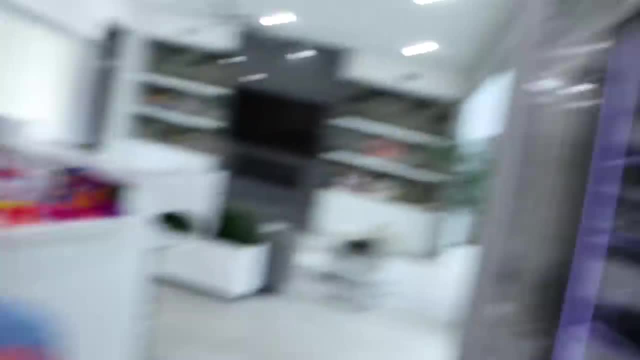 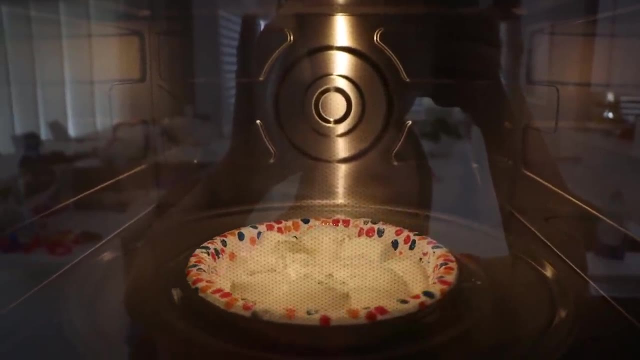 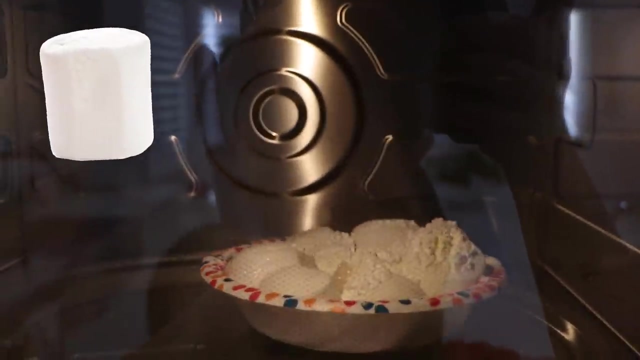 notice what happened to the marshmallows. when you microwave it, The magic's gonna happen. Well, I noticed what's happened, What It's spinning, But what's happening to the marshmallows? Did you notice it got bigger or smaller? It looks bigger, Do you see it? It's a giant size marshmallow. Oh, 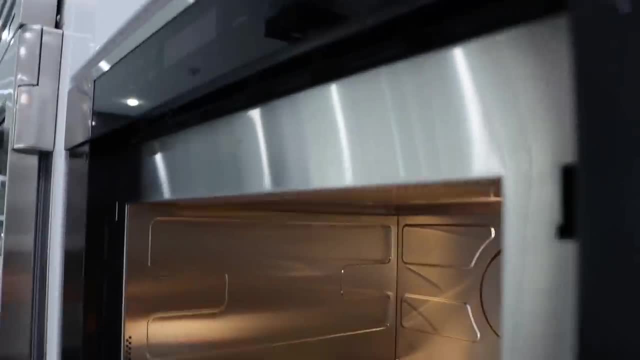 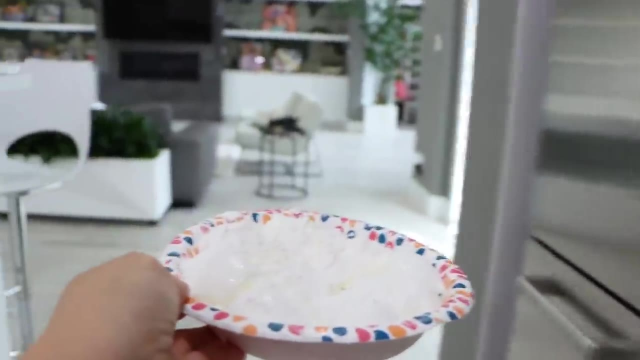 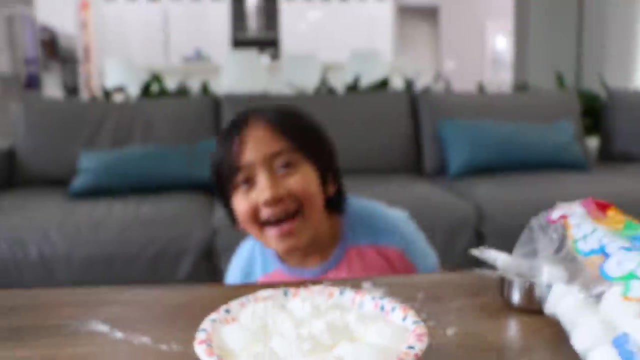 that's 30 seconds. Okay, Yeah, Okay, Look, Wow, Do you see it? Okay, Let's bring it over. It smells like s'mores. Smells like s'mores. Yeah, Next, add some food coloring. 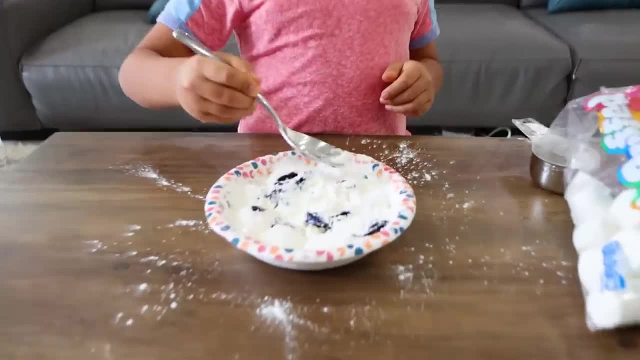 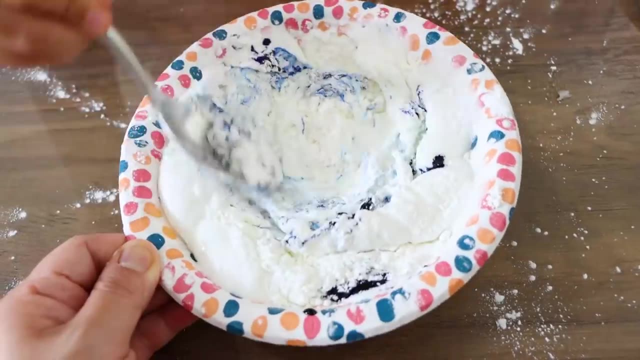 Now I'm going to agitate the blue food coloring with the marshmallows. Can I hold it for you? Whoa, Okay, Exactly like mixing s'mores. It does. huh, It looks kind of cool. Mix it all up. Mix it all up. Mix it all up, Okay. 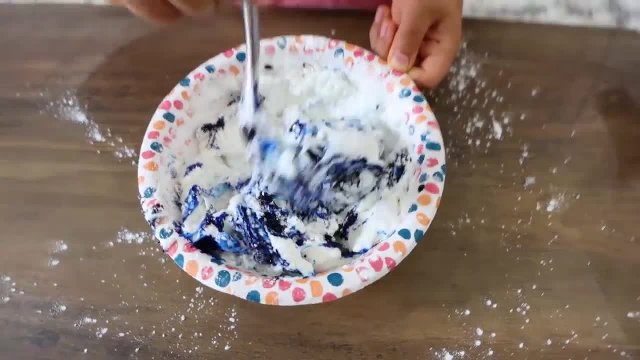 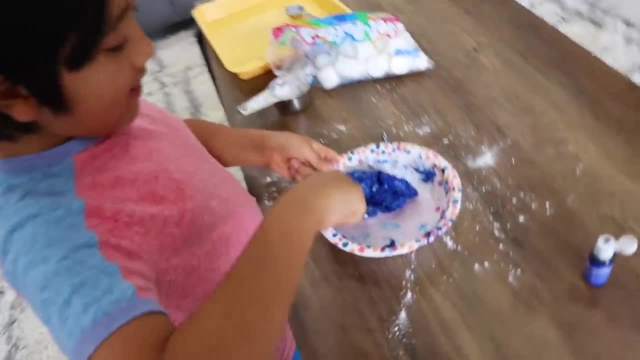 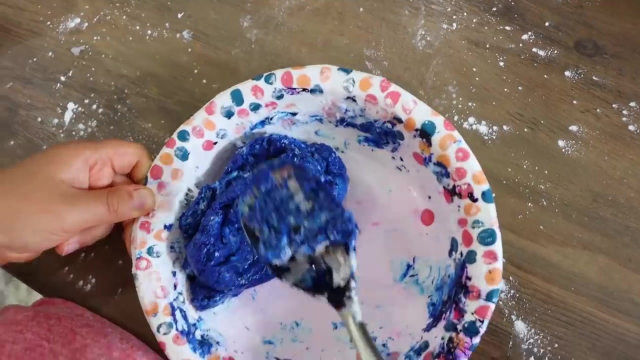 All up, agitate, agitate- What's another word for agitate? Mix Or stir. good Okay, mixing, Almost there. good job, It almost fully blew. All right. now it's a little warm, so mommy's gonna take over. 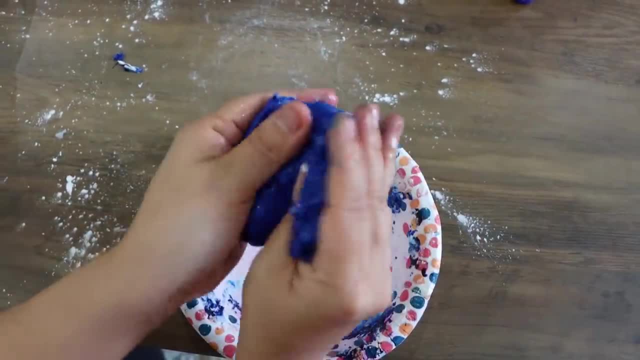 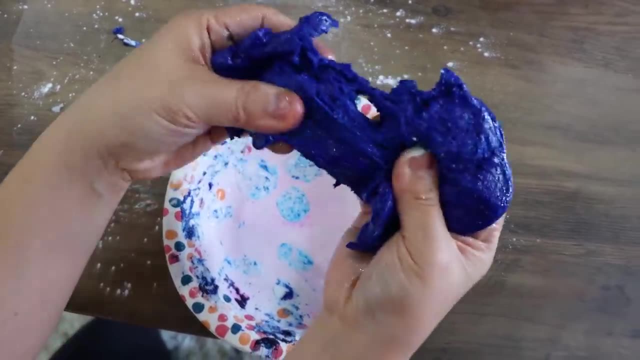 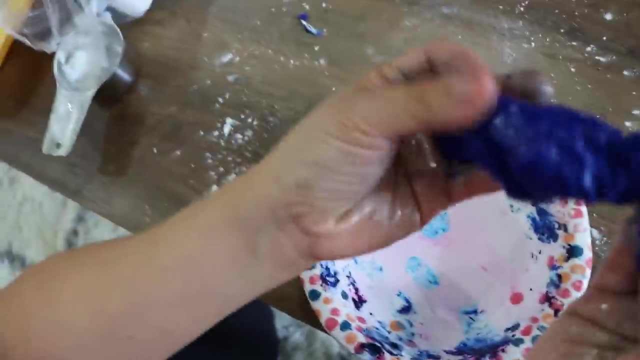 But all you do is just smush it together like so: Whee, Looks like it's starting to look like Play-Doh, Look Ooh. And then just you can even roll it and twist it, See, Woo-hoo. 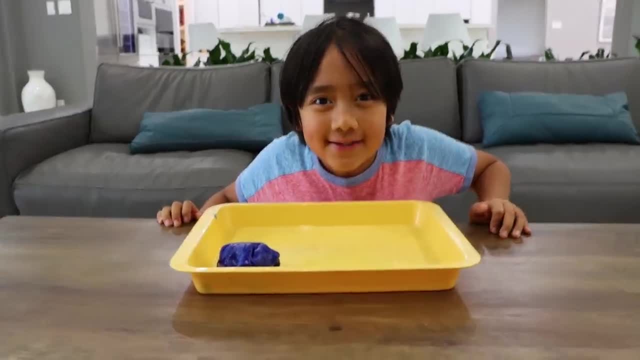 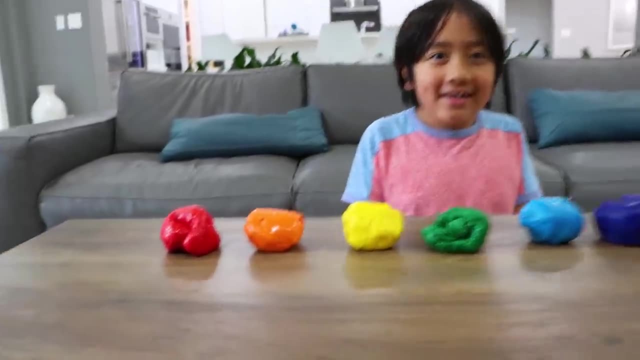 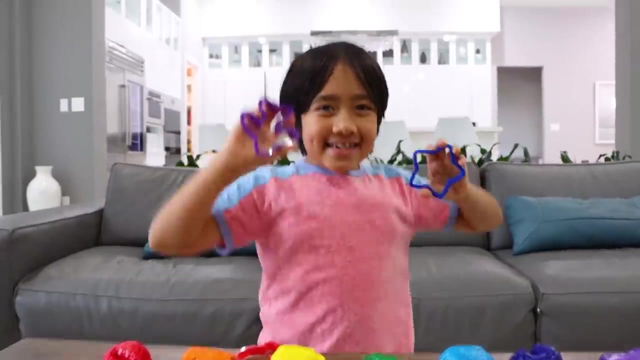 Now that we have our blue Play-Doh, let's make the other colors. Yay, we have all the colors of the rainbow of Play-Doh Marshmallow. Now Let's test it out. Okay, so first we're gonna just use orange. 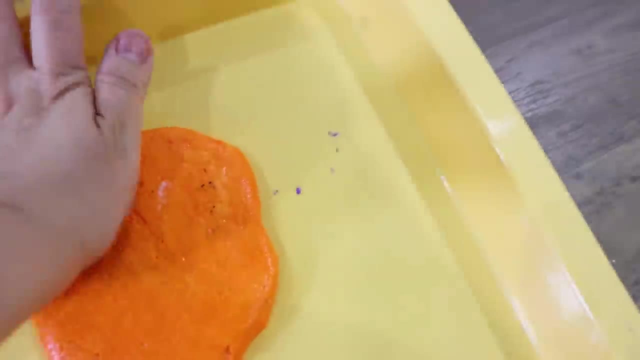 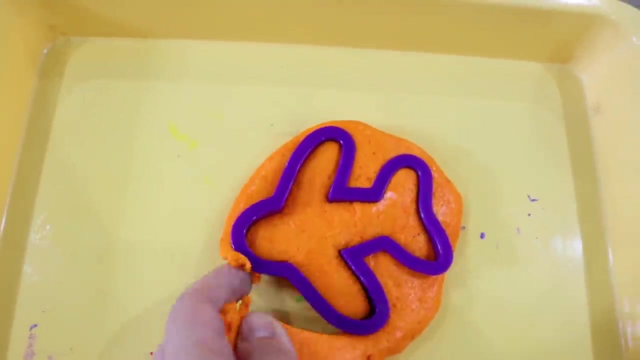 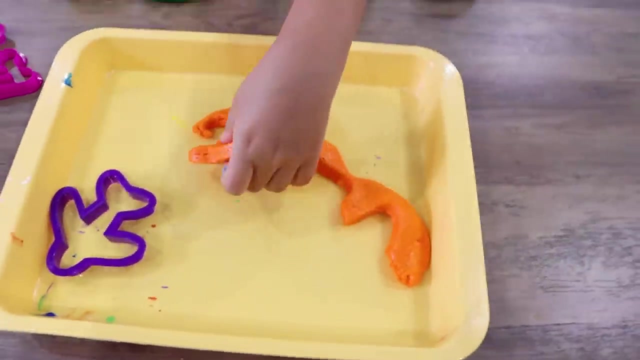 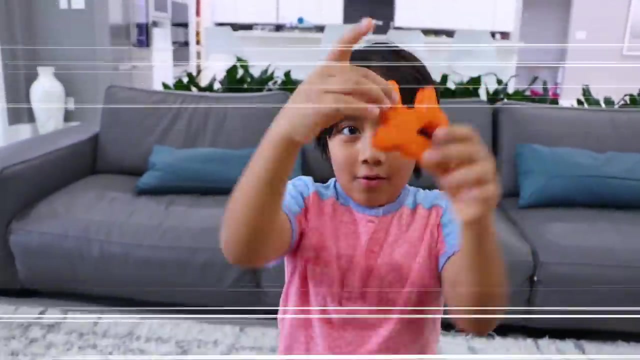 and you just press it down, Okay, And then you put it in: Okay, and now we're gonna take out the sides. Okay, Yay, now we have an orange Play-Doh. Where you going? where you going, Oh, whoa. 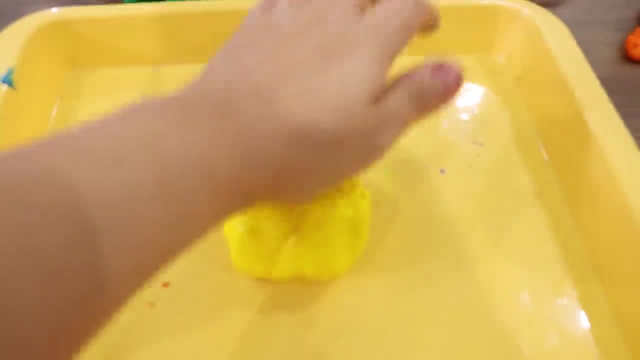 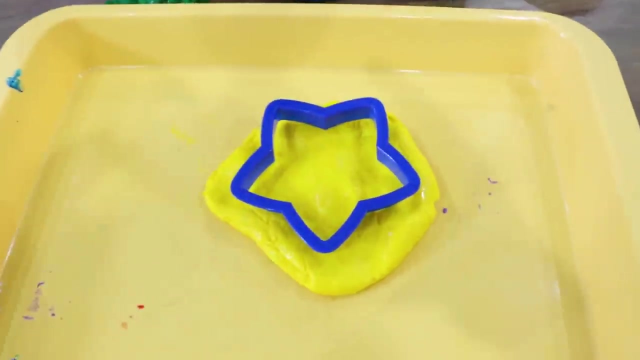 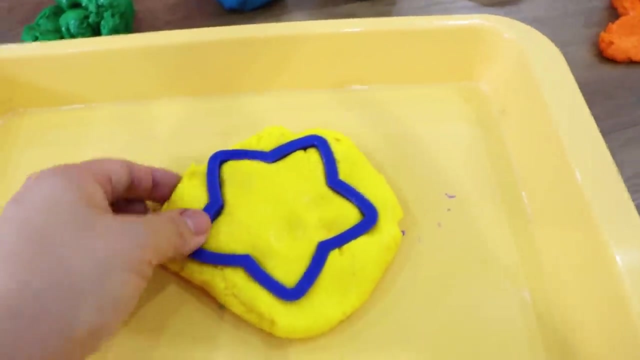 Ah, watch out. Okay, now let's see if we can make a star. Okay, let's see if that fits. Okay, and yellow star: Okay, push it in. Nice Teamwork, Can you hold this down? 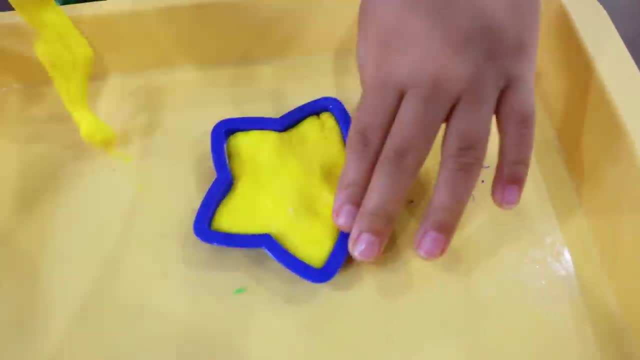 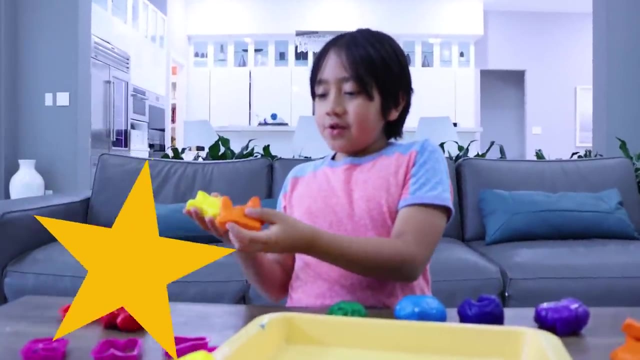 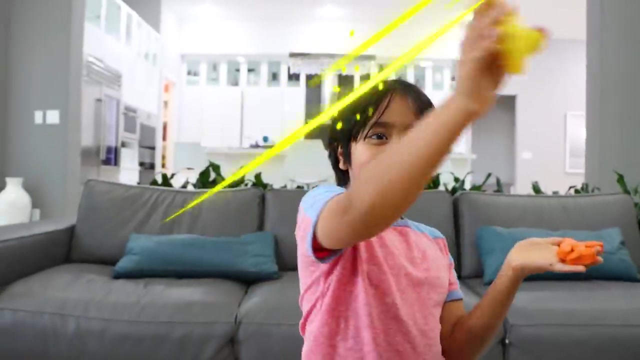 Here we go, Lift up the outside layer and bam Bam, we got a star. Twinkle, twinkle little star. How, I wonder what you are. Star plane, What do you guys wish for? Shooting star Woo-hoo. 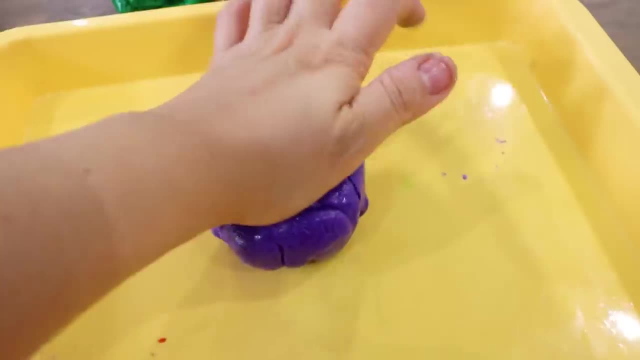 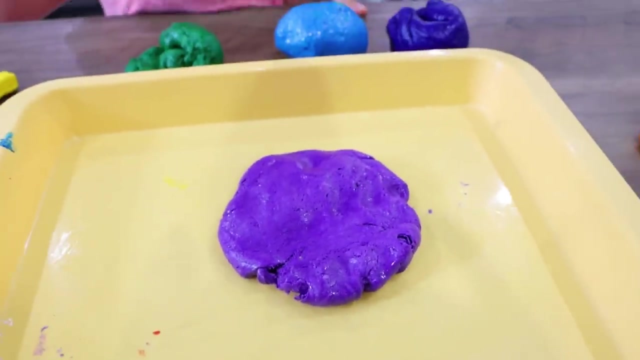 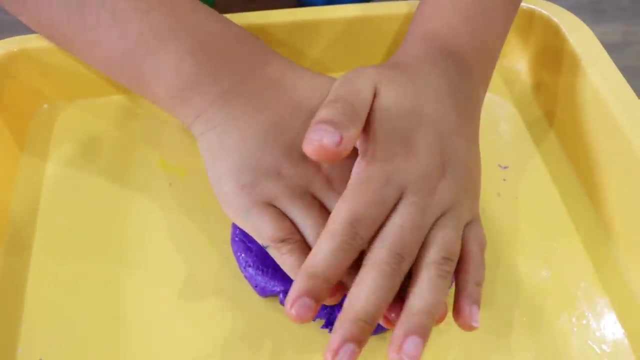